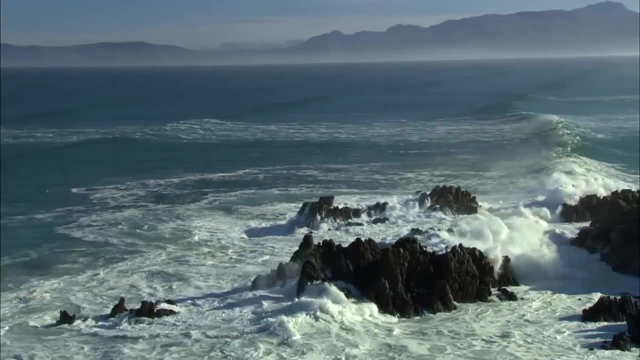 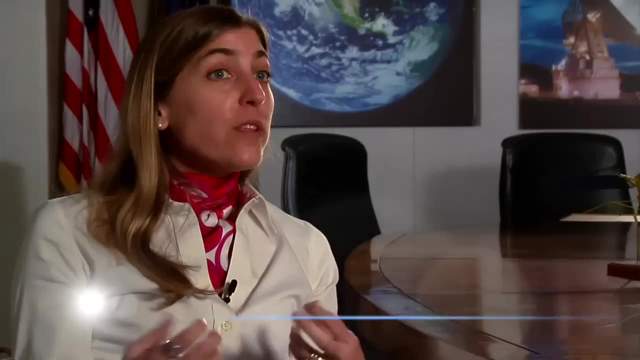 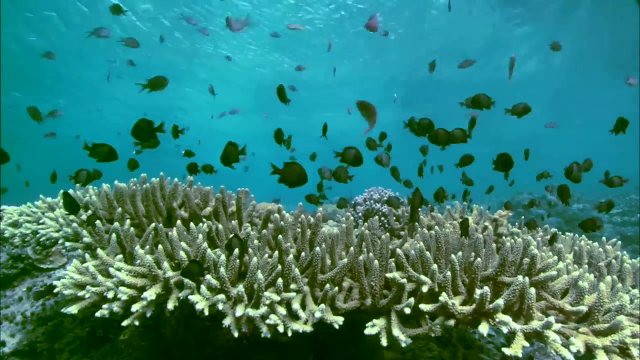 as huge, as deep, as mysterious as our oceans. Earth scientists are determined to find out. You can see the atmosphere, you can see the land, but you can't really see beneath the ocean's surface. And so you start wondering. you know what's going on beneath the part. 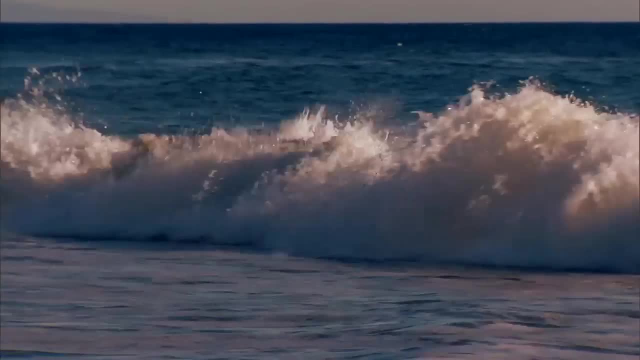 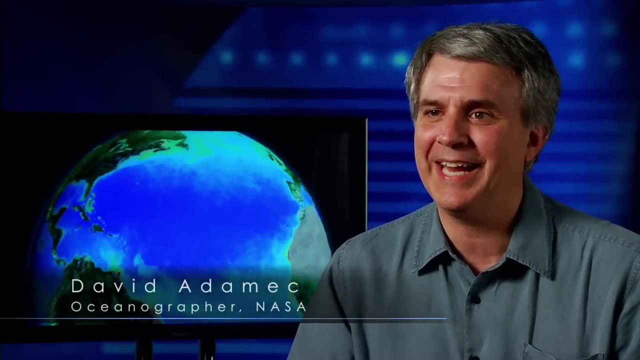 that we can see. We walk in a very small part of the atmosphere and we walk on the land, and it's how that interaction takes place with the ocean, the atmosphere and the land that determines, you know, our quality of life. Our goal is to understand the interconnectedness. 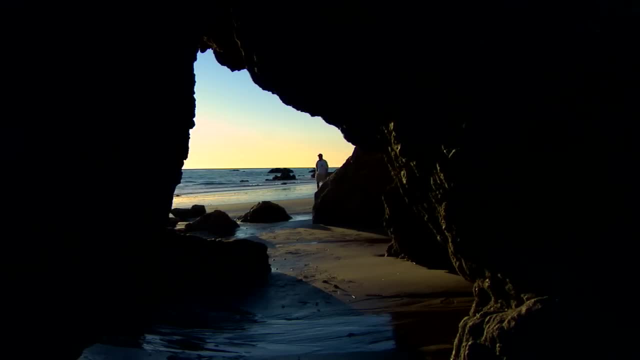 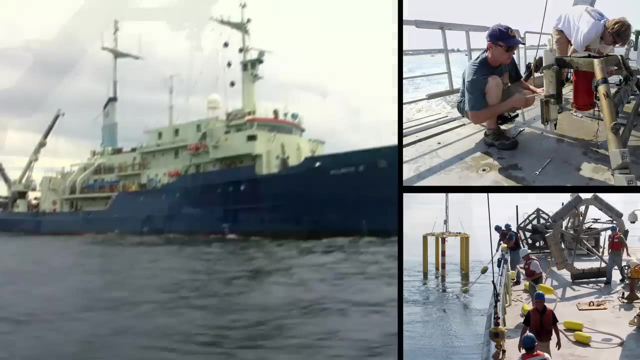 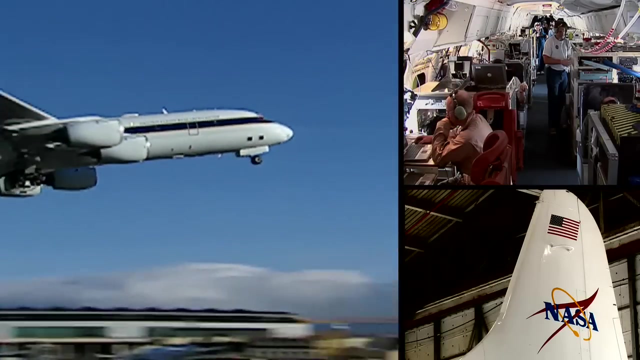 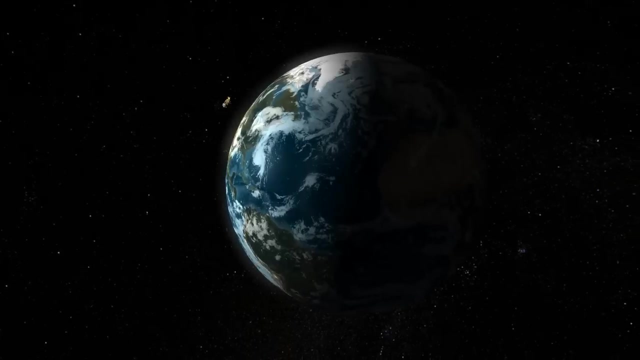 of it all. For years, people have worked to unravel the mysteries of the oceans. Scientists gather data from ships and buoys on the surface, Take the plunge to explore ocean depths and fly overhead to get a bigger picture. But one of the best views of oceans might be from way, way overhead. It's the view from 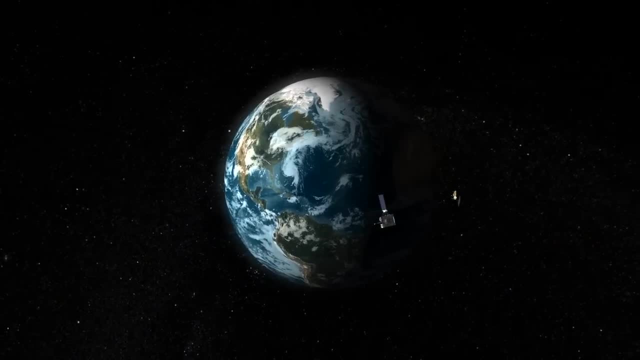 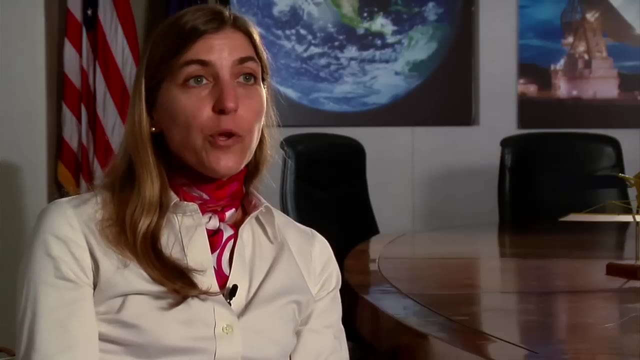 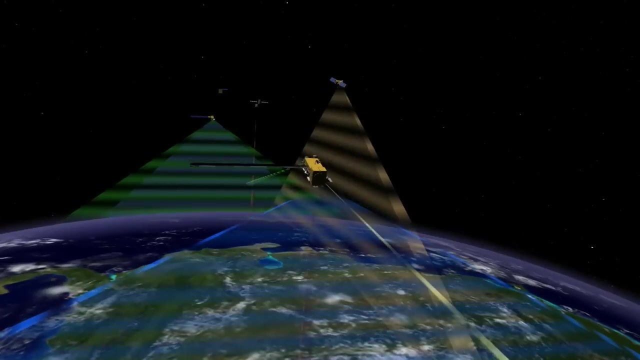 space. The one thing that NASA satellites do that nothing else does- ships or buoys or anything else- is actually give you a picture of the globe within a few days. You don't get a much broader view of what's going on in some part of the Earth system and you 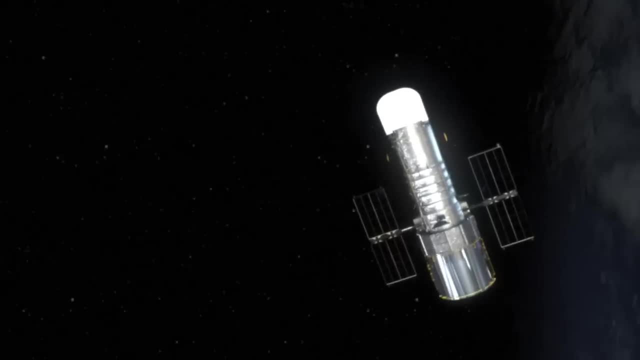 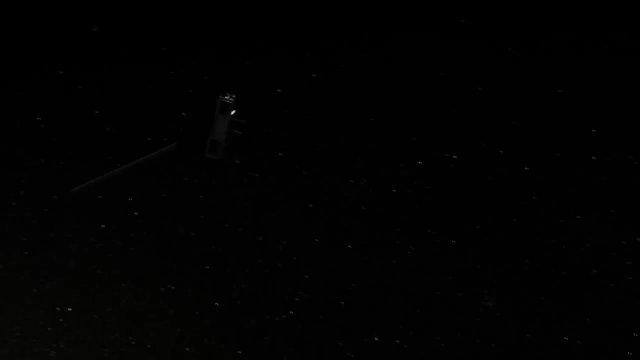 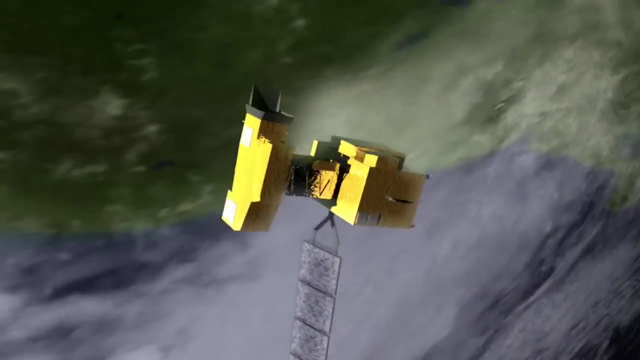 can link that together to understand the Earth as a whole. Thousands of satellites orbit our planet. Some look out into space, Others look back at us at Earth. Some of the sensors on these satellites act like giant digital cameras taking pictures in visible light, the kind our eyes see On land these images show us. 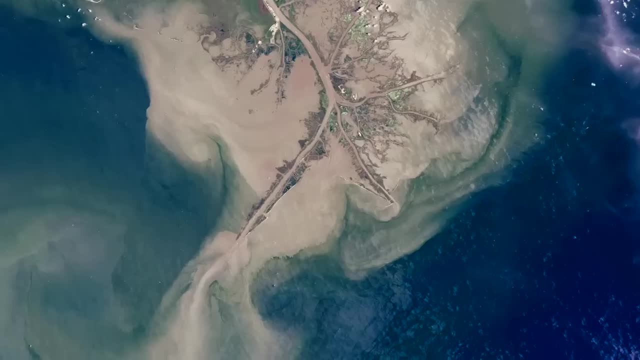 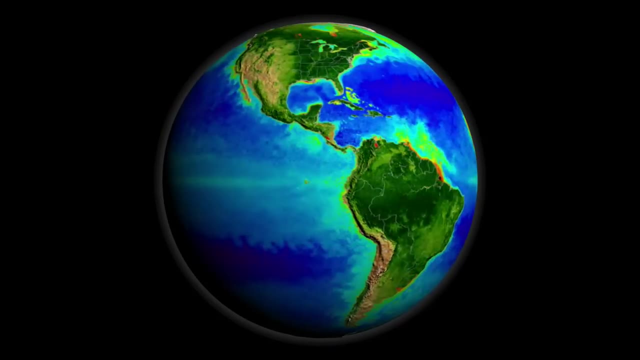 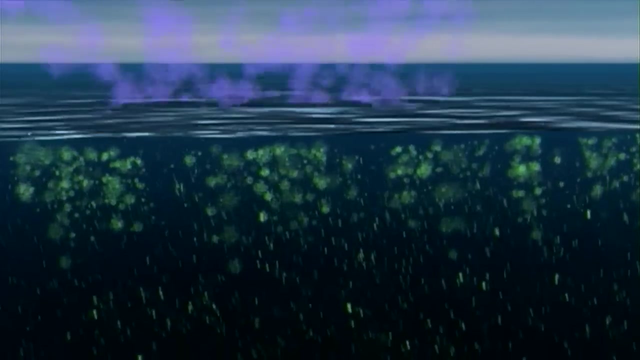 when plants turn green. They help us see where dirt and pollution drain into the sea and where microscopic plankton thrive. These tiny organisms are not only the base of the marine food web. they give us the air we breathe. We are dependent on life in the water, especially in the ocean. There are small plants called 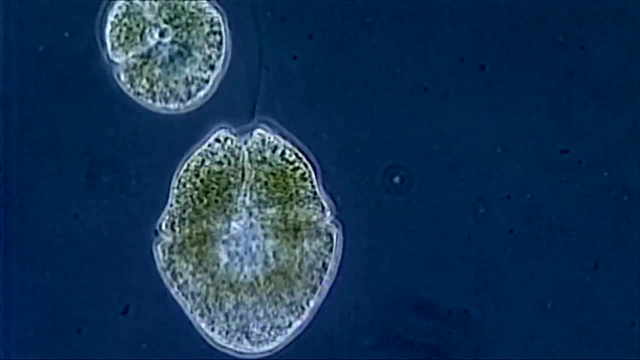 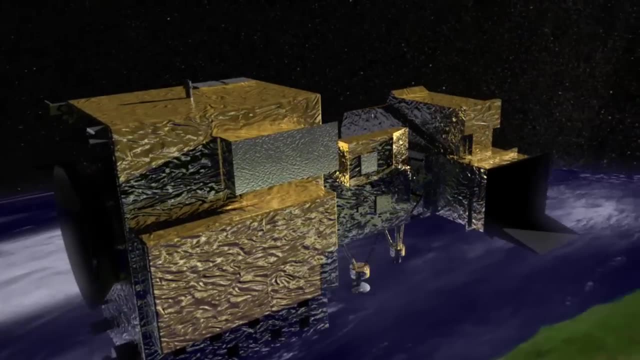 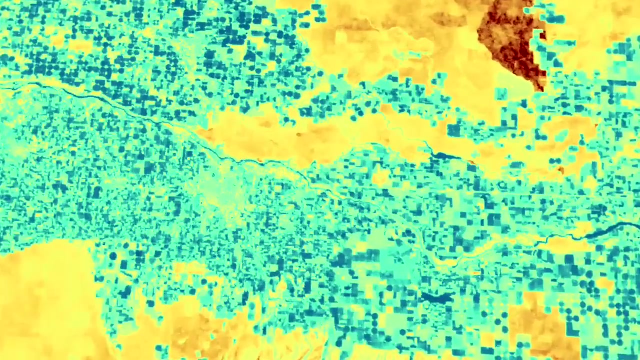 phytoplankton that are responsible for 50 percent of the oxygen that you're breathing right now. Other kinds of satellite sensors look at the Earth in a far different light. Heat-sensing satellite instruments take the Earth's temperature by measuring infrared energy, Infrared wavelengths.